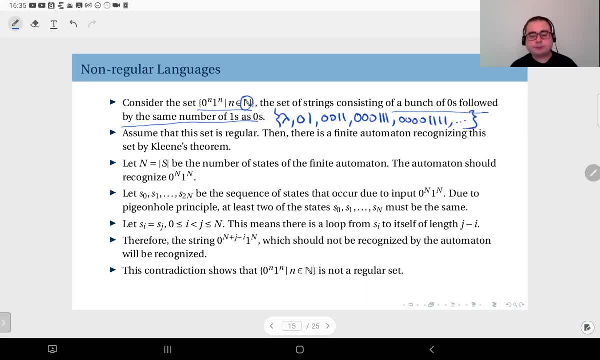 1, 1, 1, 1 and so on. The question is: is there a regular expression to express this set of strings? Now, let's assume there is. Assume that this set is regular, Then this means there is a finite automaton. 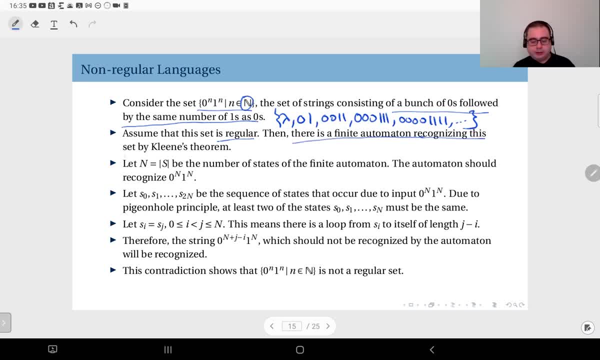 by Killeen's theorem. There is a finite automaton recognizing this set. And again, remember, this is a finite automaton, So it has finitely many states. Let's assume the number of those is n And since n is a non-zero integer, 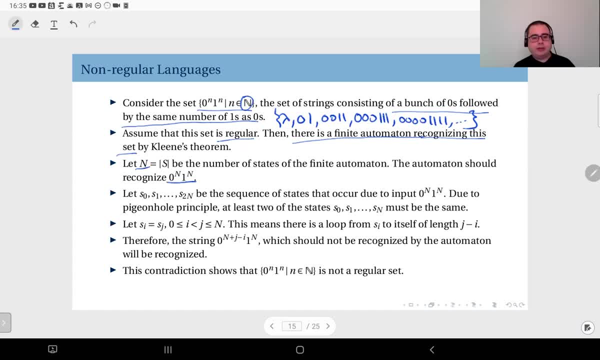 the automaton should recognize the string 0 to n. 1 to n, meaning that you have n zeros followed by n ones. Now consider the states that the automaton passes through while recognizing the input 0 to n. 1 to n. 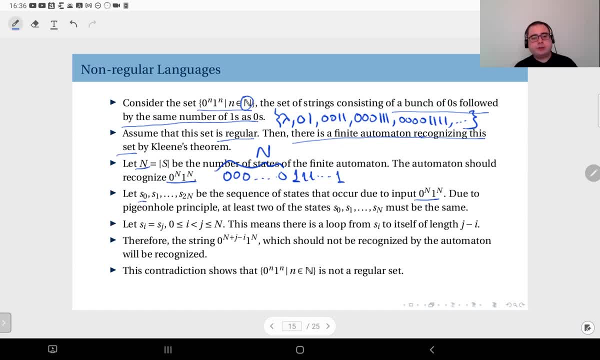 Let's say these are: s0, the initial state, followed by 2n states in recognizing this string, because we have assumed that it should be recognized by this automaton, Now consider the first n plus 1 states: s0,, s1, up to sn. 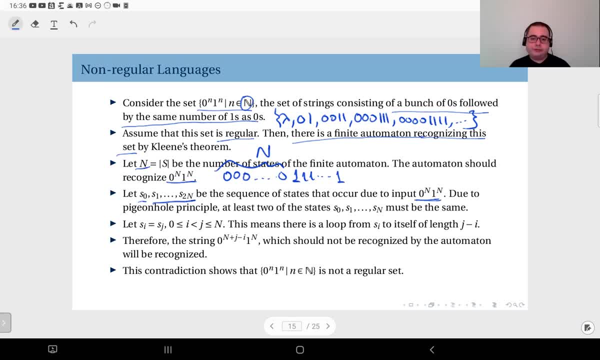 Now, sn is the state we reach after the last 0, before the very first 1.. This is the state we reach, So s0 through sn. Now there are n plus 1 states here And by the pigeonhole principle, recall. 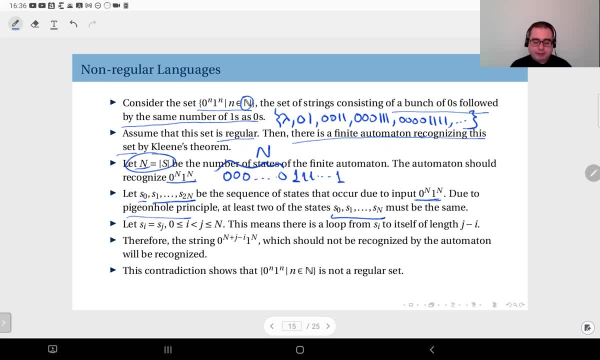 since the number of states is n and I have n plus 1 states in this sequence, at least a pair in the sequence must be the same, So I must have a repeated state here in this list, Assume that those are si And sj. 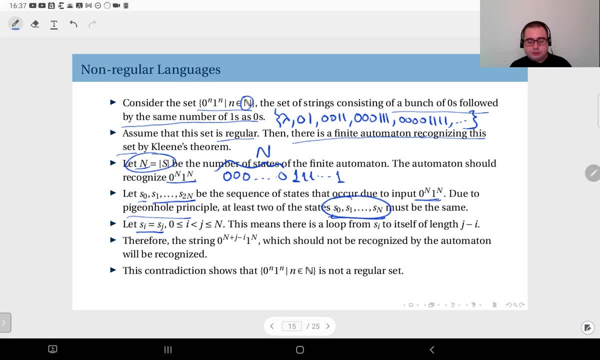 And i and j are between 0 and n, obviously inclusive, But assume that i is less than j. This is strict inequality here. i less than j and not equal. That is essentially due to the pigeonhole principle. We have established that at least two different states. 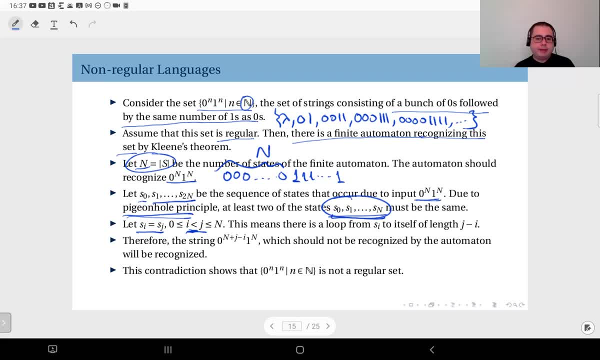 here must be identical, because we have n plus 1 states in this sequence, But the total number of states must be the same. So we have n plus 1 states in this sequence, but the total number of states is n. So this means there is a loop from si to itself, which is sj. 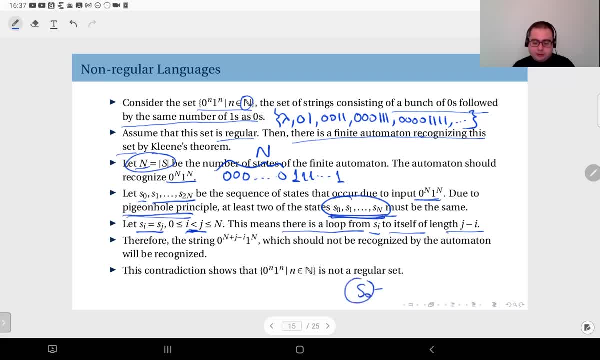 of length, j minus i, So you have s0,, s1, and with all 0s you end up with si, And there is a loop to itself, because at step number j you are also at si, And then you continue to sj plus 1, and up to sn. 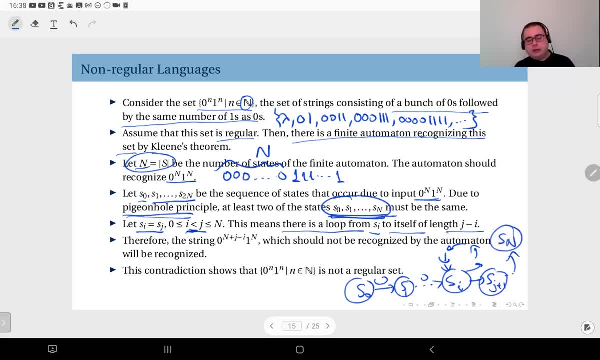 So this means there is a loop of length j minus i, And j minus i here is not 0. It's positive. Now consider the string 0 to n plus j minus i, 1 to n. So this means you have n plus j minus i, 0s followed. 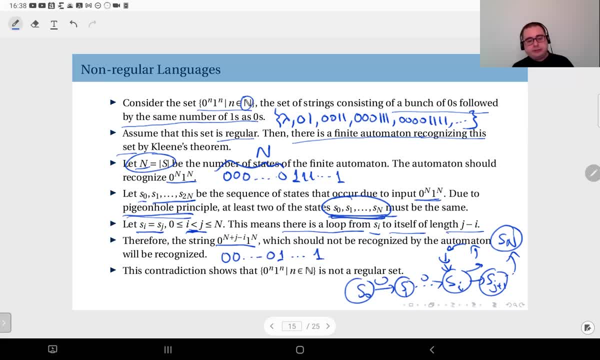 by n- 1s. Now this doesn't fit the description given here- 0 to n, 1 to n- because it doesn't have the same number of 0s as 1s, So it should not be recognized by the finite automaton. 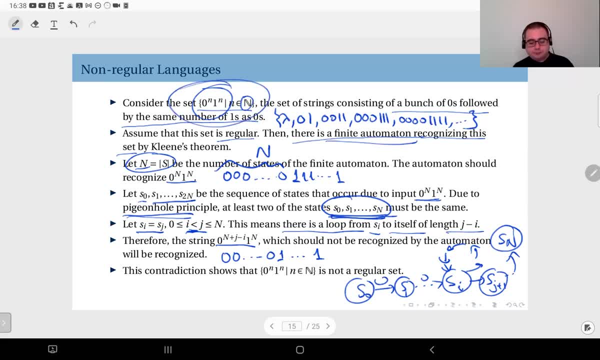 recognizing this language here. However, since I have a loop from si to itself of exactly j minus i length, This string will also be accepted, because when I hit si, I'm going to take a loop of j minus i And, due to this excess, j minus i. 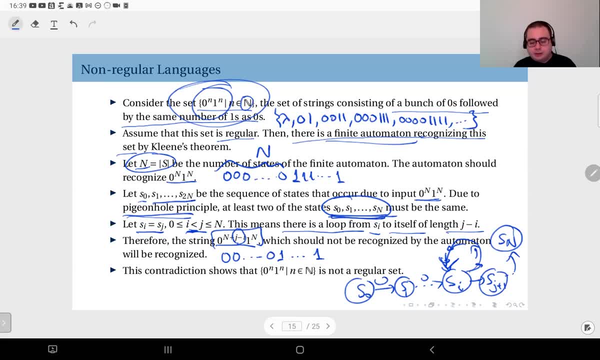 I'm going to take another loop here, from si to itself and then continue the transitions, which will follow the same exact path that the input 0 to n, 1 to n caused. So the result will be an accepting state, which means this string, which is not in this form: 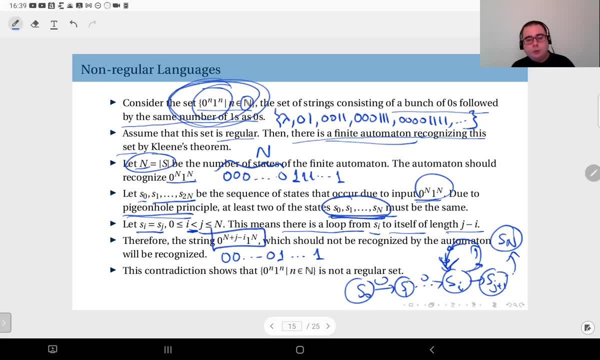 is going to be accepted by this finite automaton which leads to a contradiction. Therefore, this cannot be a regular expression, It cannot be a regular language. Alternatively, we can say that there can be no expression. It cannot be a regular language. 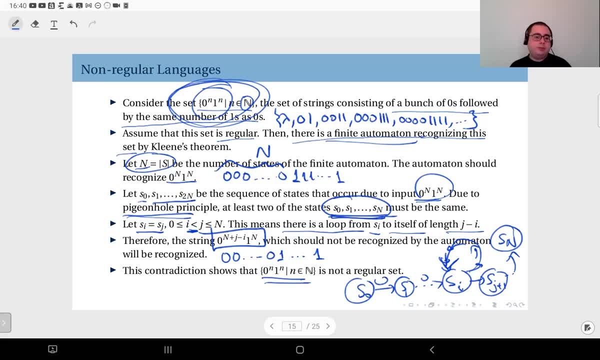 Alternatively, we can say that there can be no deterministic finite automaton or non-deterministic finite automaton that recognizes such a language. That is due to the fact that the finite automaton has no infinite memory, Because n here the number of 0s or the number of 1s. 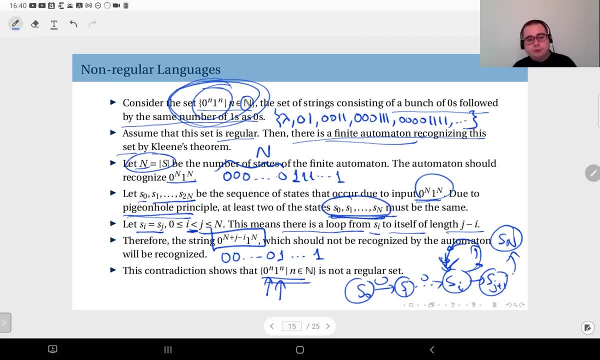 can be arbitrarily large. So for the recognition of such a string you have to remember how many 0s you encountered And you cannot really set aside a different state for counting the 0s, because however many states you define, there can be a longer string that your machine will. 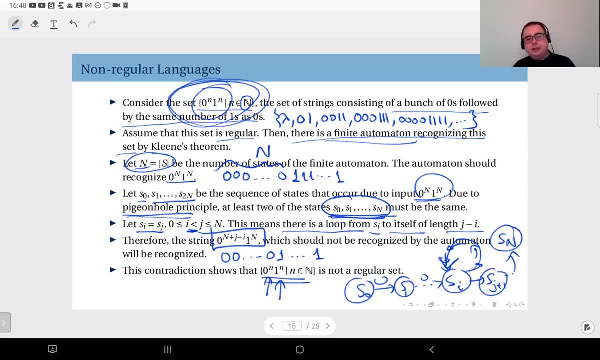 be unable to recognize. Therefore, the fact that your finite state automaton has memory embedded only in the states and the number of states is finite, such a language cannot be recognized by a finite state automaton. Therefore, this is not a regular language. 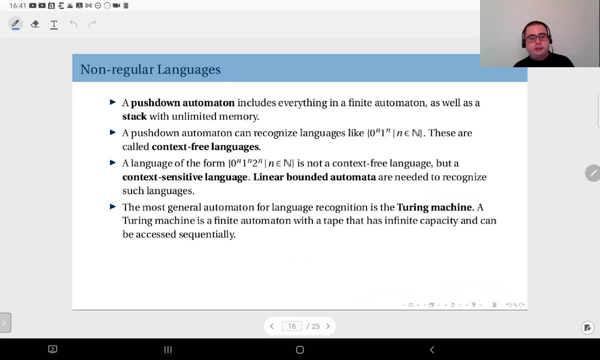 So what to do? How are we going to actually recognize such languages? To recognize such a language, we have what we call a push-down automaton. Now here, the difference from the finite state machine or the finite automaton is it includes everything. 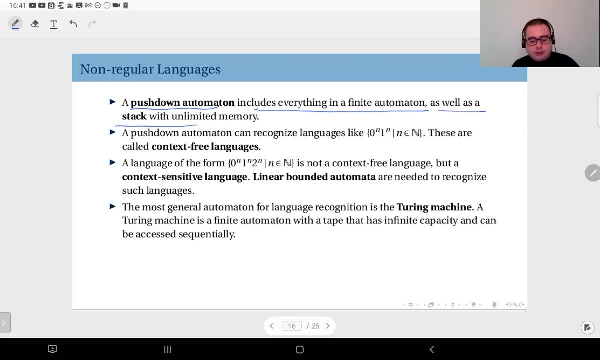 in a finite automaton. It includes everything in a finite automaton, as well as a stack with unlimited memory. Now you have a separate memory unit. apart from your states, You have a stack, so you can push and pop values to your stack. 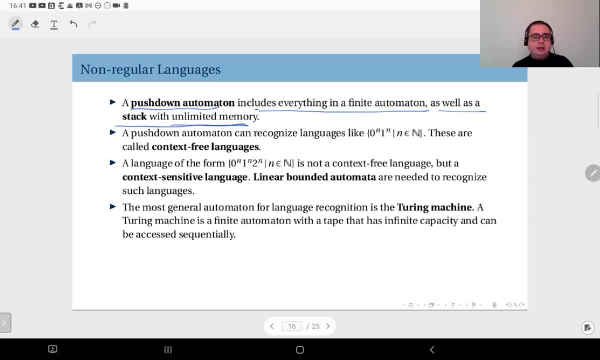 And essentially, the capacity of the stack is not limited. So that is how you come up with a structure that can recognize such languages. So what are you going to do? As long as you encounter zeros, you are going to push them to the stack. 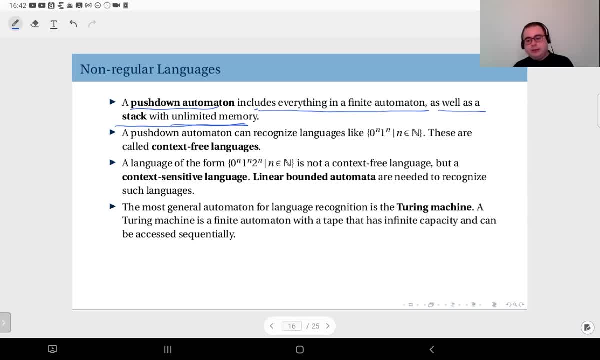 And when you start seeing the ones, as soon as you encounter one, you pop one of the zeros. With another one, you pop another zero With another one, pop another zero, Of course, along the way, if the pattern is spoiled. 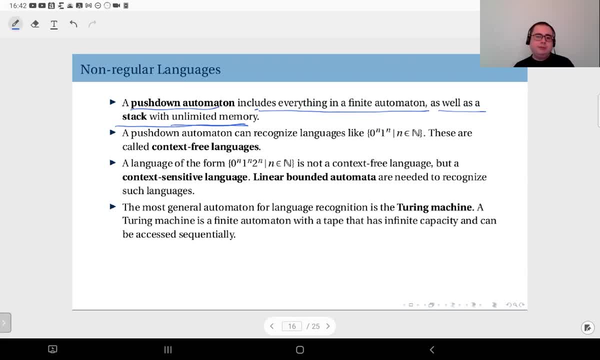 then you give up and do not accept. But if you reach the end of the string and you encounter the final one which matches the end of the stack, which you pop, the final zero, then you know that the number of zeros and the number of ones. 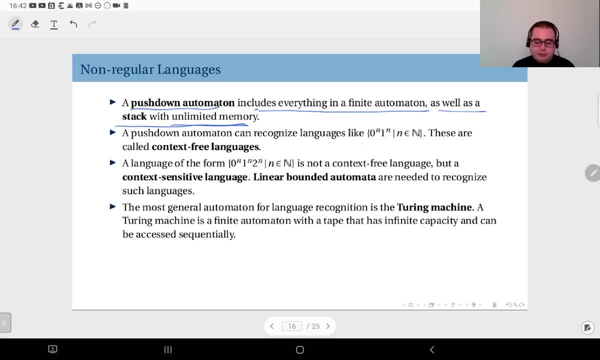 would be equal. So that is how you recognize the string 0 to n, 1 to n, using a pushdown automaton, And such languages we call context-free languages. These are a broader category than regular languages and they require able to accomplish those. But it's also possible you can use that to new things in data collection. The image you see here is a是不是 single code. Here there is a Foregroundnahal spherical listing model, a blend issue, And you can use this to calculate everything using basedogram. 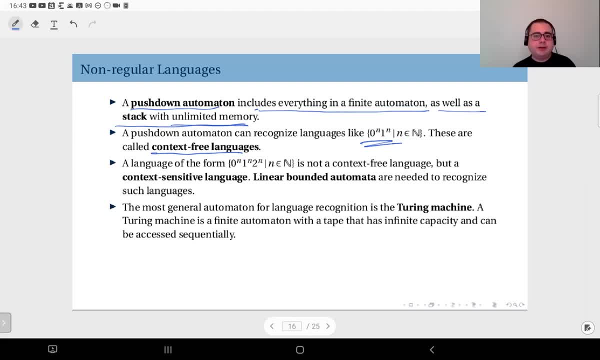 And you as a user, you create the faster known and standardized tag line 1 and Creating a spaced list of concepts such as machinery further than finite state automata. But these are not the exhaustive, let's say capacity exhaustive- category of languages We have. for instance, if you have 0 to n. 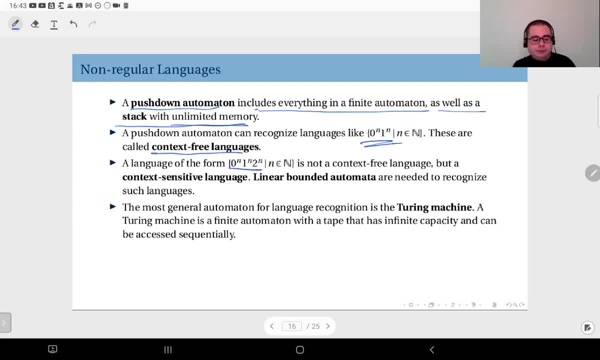 1 to n, 2 to n. let's say you have an alphabet of three symbols- 0,, 1,, 2, and using a pushdown automaton it is not possible to recognize such a language. I'm not going to go into the details. 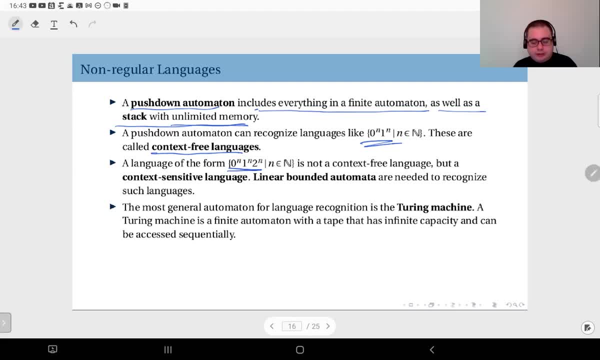 but essentially you can show that such a set is not a context-free language, but it's a context-sensitive language, Because the number of ones depends on how many zeros you encountered before and how many twos you'll encounter later on. So this is what we call a context-sensitive. 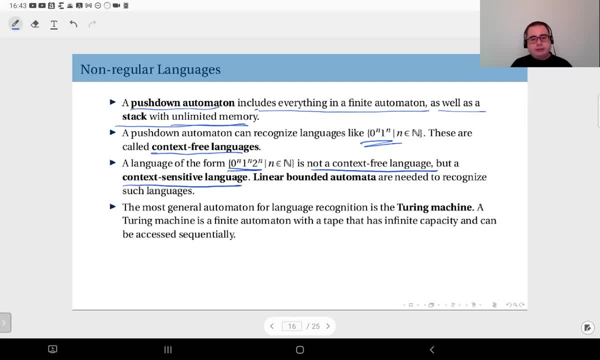 language. To be able to recognize such languages, we need linear bounded automata. Okay, so this is a more general structure than the pushdown automata And, again, I'm not going to go into the details of this, but these are important concepts when designing. 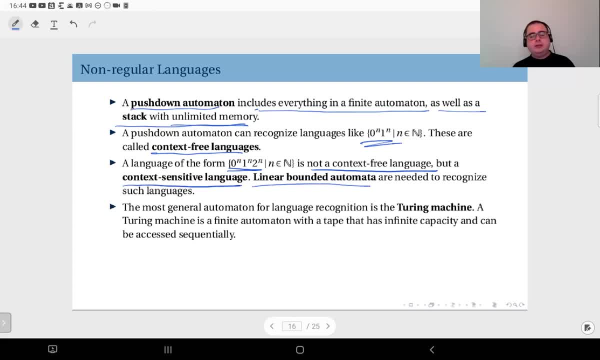 programming languages, essentially And again. furthermore, context-sensitive languages again, are not the most general case. The most general case in the theory of computation is for language optimization. The most general automaton is the Turing machine. A Turing machine is a finite. 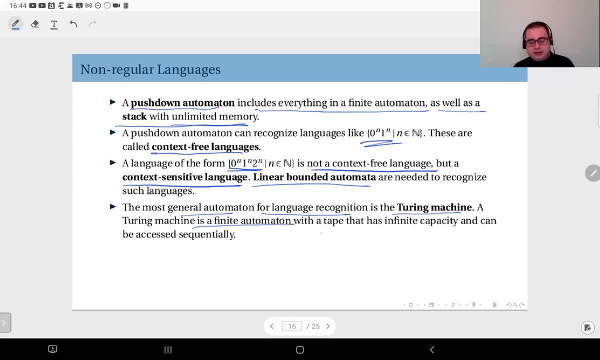 automaton along with a tape. So you have a memory that you can read and write, and it has infinite capacity and you can access it sequentially. So you have a tape, potentially with data on it when you start your program. So that is the string, let's say, to be recognized. 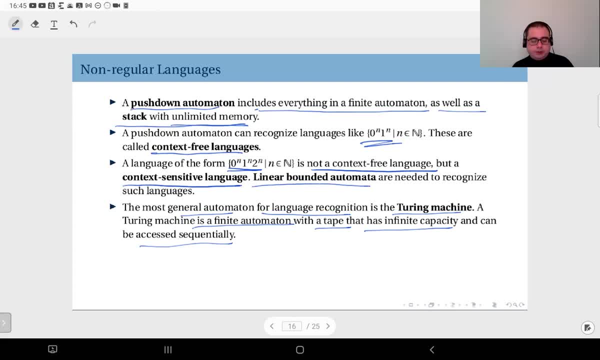 And the tape can move towards right or left so that you access every symbol And you can modify whatever is written on the tape, depending on your state and the symbol on the tape. You switch your state and you modify. you possibly modify- you don't need to, but you can modify the. 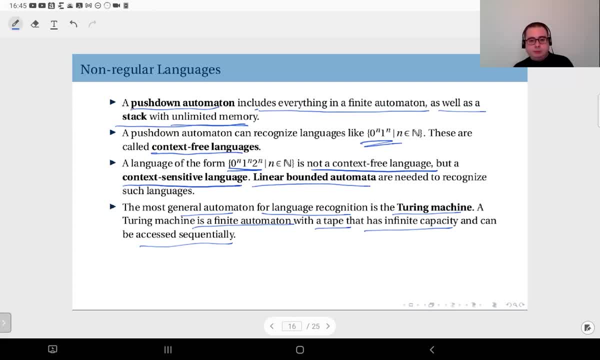 symbol on the tape And you can modify the symbol on the tape. you can modify the symbol on the tape, symbol at the current position in the tape, and then you move one position towards right or towards left. So that's essentially what we call a Turing machine and it is the most. 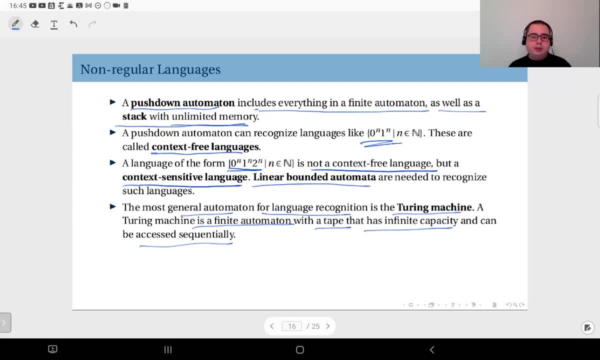 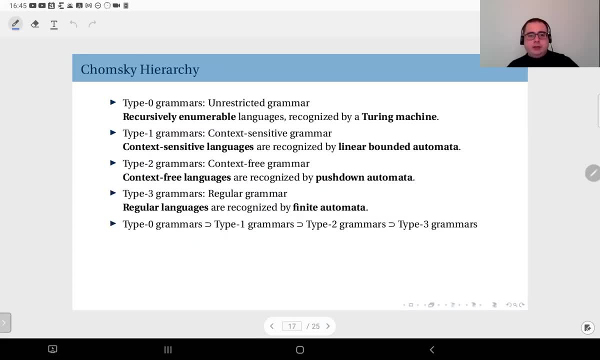 general computational tool in the context of theory of computation. And these languages, they define the hierarchy, as you have seen, and the type 0 grammars are unrestricted And we call these recursively enumerable languages and this is an important concept. in mathematics also, We have the concept of recursively enumerable functions and these are recognized by a Turing. 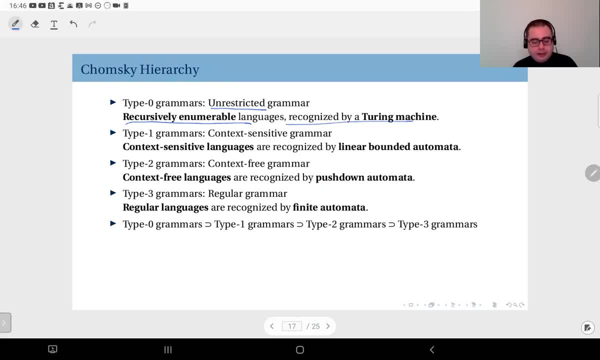 machine. it's possible to prove this And if you go one step further, you might see that there is also an enumerable function called the Turing expression. it's called in special considerations. you have type one grammars. These are context sensitive grammars.